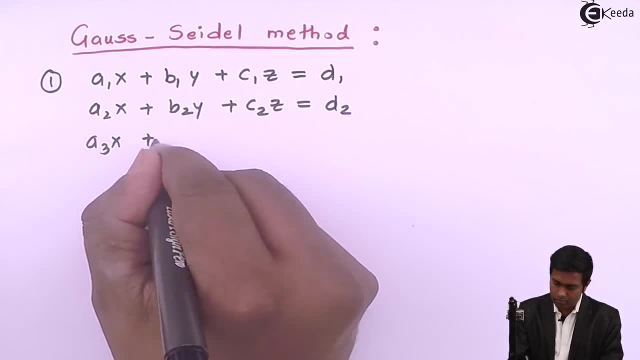 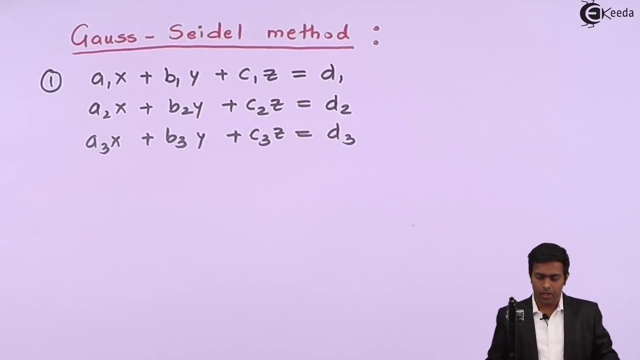 a2x. Now let us say we have three simultaneous equations with three unknowns. Now to get the roots of these three equations. if you will observe, then coefficients a1, b2 and c3 will be large as compared to other coefficients of x, y and z. 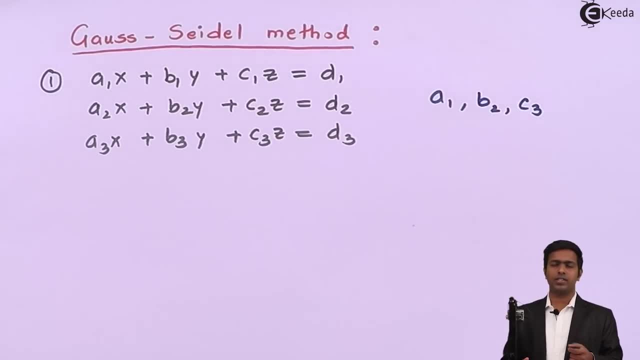 So if we want to solve this equation by Gauss-Siedel method, then we will first of all represent these three equations in such a way that these large coefficients will go in the denominator. So see here how I am representing. So I will represent this first equation as x equal to 1 upon a1 into d1 minus b1y minus c1z. 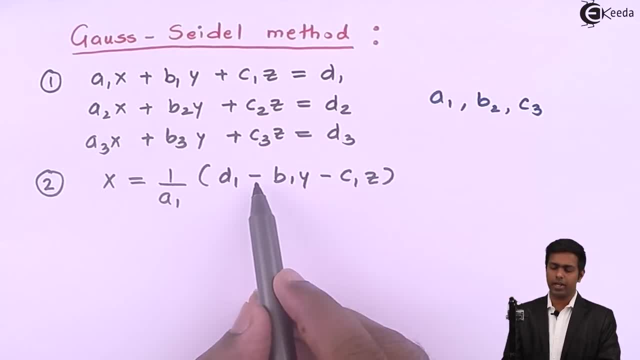 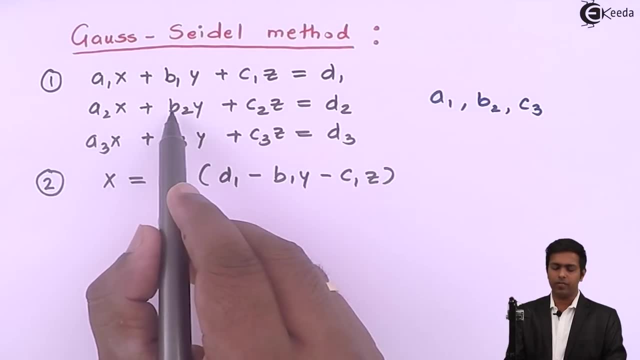 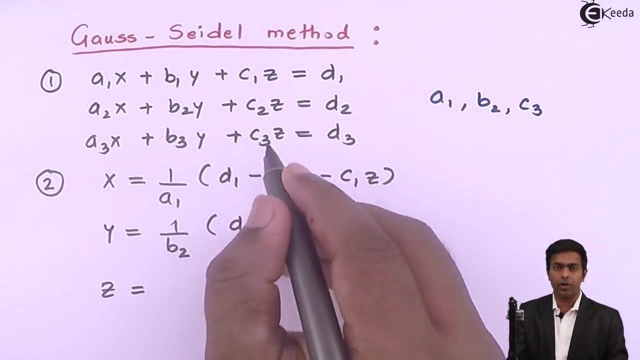 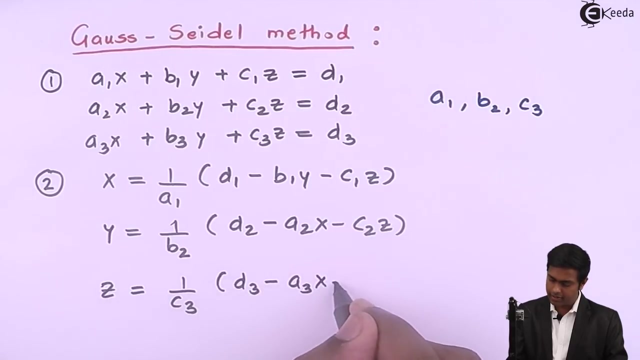 So I am taking this b1y and c1z. on the other side that will become negative And this a1, which is multiplying x, will go and divide there. Next from second equation we have b2.. So I will say y is equal to 1 upon b2 into d2 minus a2x minus c2z, and z equal to 1 upon c3 into d3 minus a3x minus b3y. 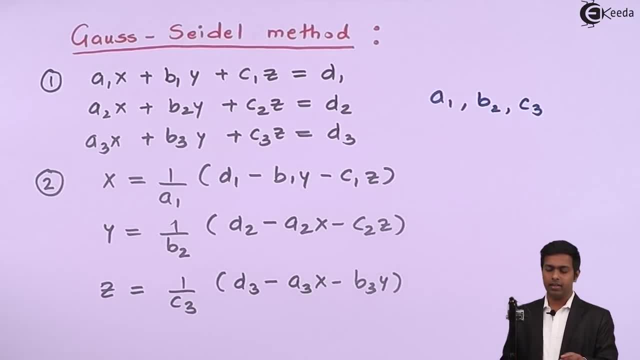 So here we will get the value of x, y and z. Now to get the roots of the equation, we will use the method of iteration, because Gauss-Siedel method is the iterative method. So what is iterative method? So here we go through multiple iteration or multiple rounds and we come closer to the roots. 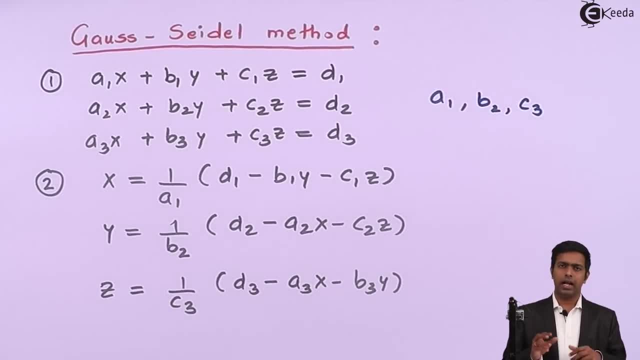 And once we get the desired accuracy of the root, that is our final answer, or that is the root of the equation. So to reach the desired accuracy or the proper root of this equation, we have to start with certain roots. So here we start with certain assumptions. 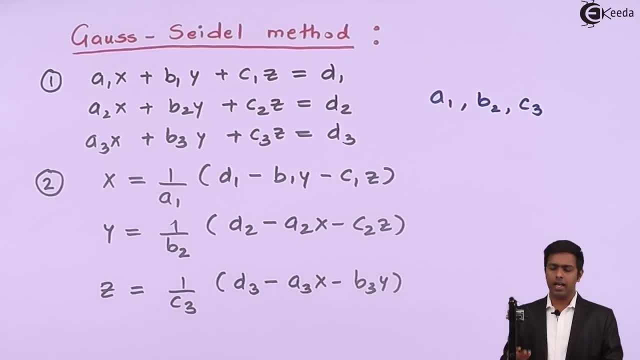 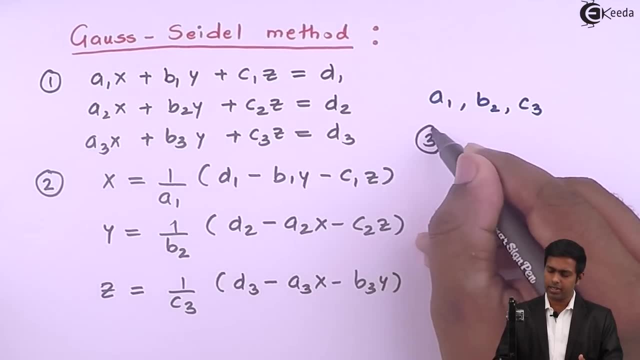 So we say that initially the roots of the equation at, So I will assume that initial root of y and z as 0. So here in step number 3, I will say: put y0 equal to 0 and z0 also equal to 0. 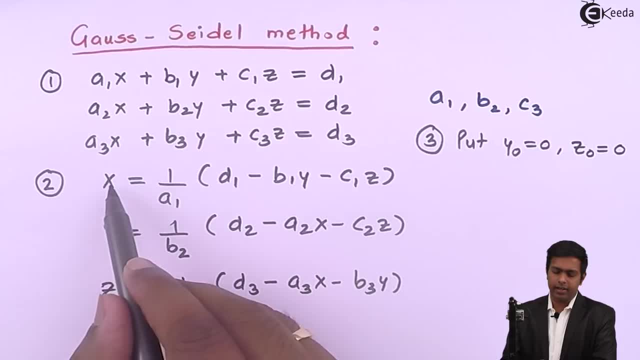 So by substituting it as 0, you will get x1 as d1 upon a1.. So see, I am starting with first iteration. So here the initial roots will be called as 0. Then the next roots will be called as 1, 1, that is, x1, y1, z1, then x2, y2, z2, x3, y3, z3, and so on. 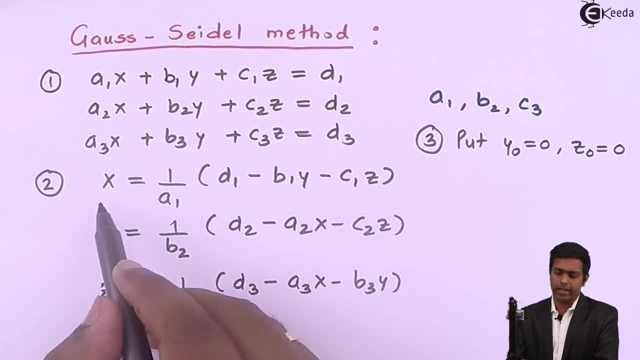 So when y0 and z0 are 0, we are getting x1. that is the next iteration, So it will be d1 upon a1.. Now, as soon as we get any new value, so this is the new value of x. 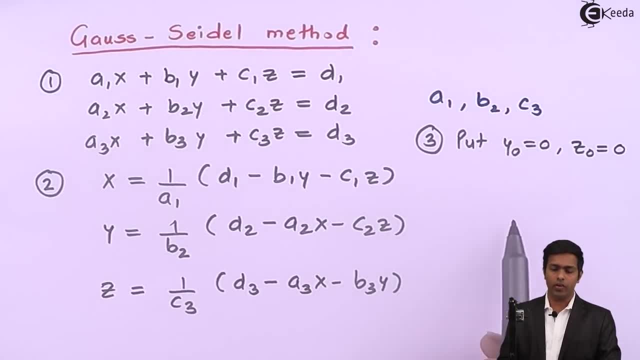 In the next equation we will use that new value, And this is the major difference between Gauss-Seidel method and Jacobi's method. So in Jacobi's method what we do is we consider the initial roots as 0, 0 in case of y0, z0 and also for x0.. 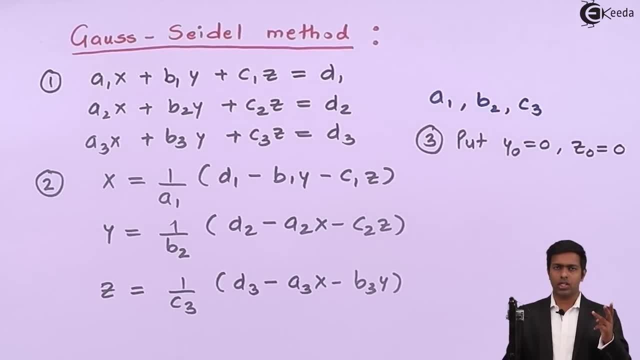 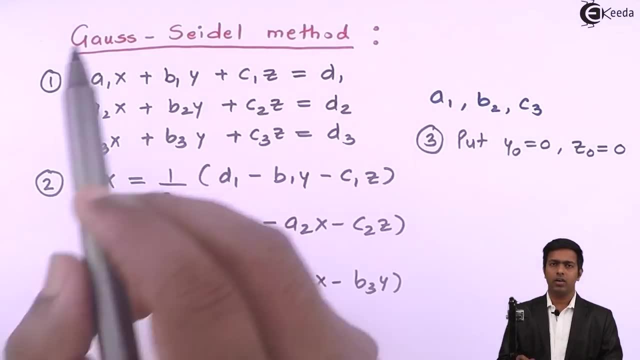 So we consider all three roots as 0. Then we find out x1,, y1, z1 and we put it in the next iteration. But here in Gauss-Seidel we just consider y0,, z0,, 0 and we find out the value of x1.. 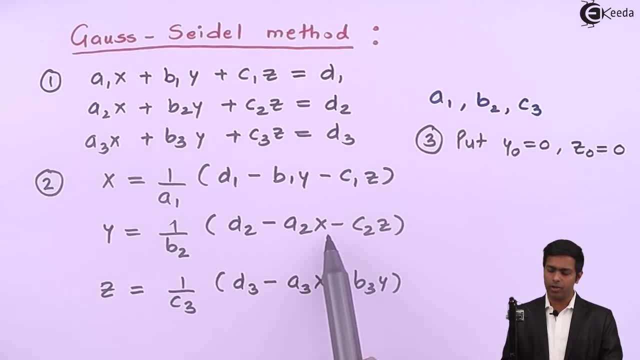 And immediately in the next calculation. we are going to use the value of x1 here, because x1 is the latest value And z still. we do not have latest value, So we will be using the same root of z0, that is, 0.. 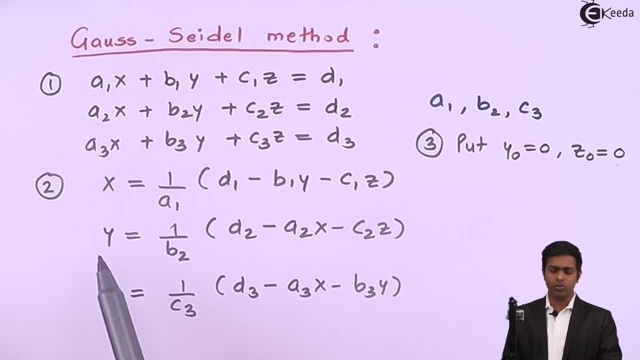 So we will get y1.. As soon as we get y1, we will use that value of y1 in the next calculation. So here y1 is the latest value. Similarly, the latest value of x is x1.. So I will use x1 here and we will get z1.. 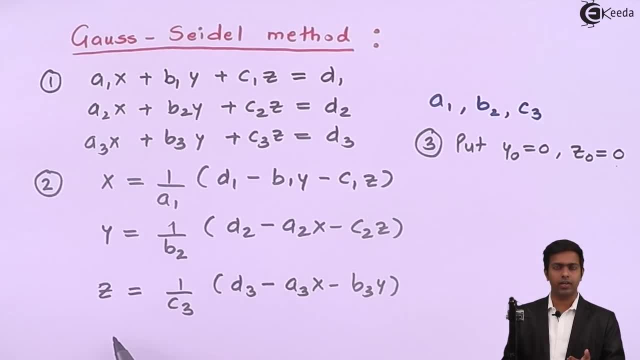 So after the first iteration we will get x1, y1, z1.. Now, while going in the second iteration, we will find out the value of x2 by considering y1 and z1.. Next, y2 by considering z1. 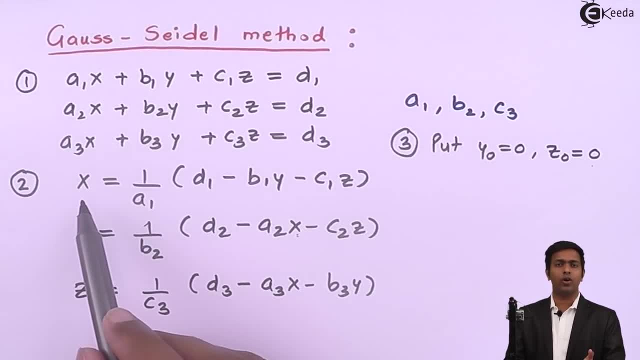 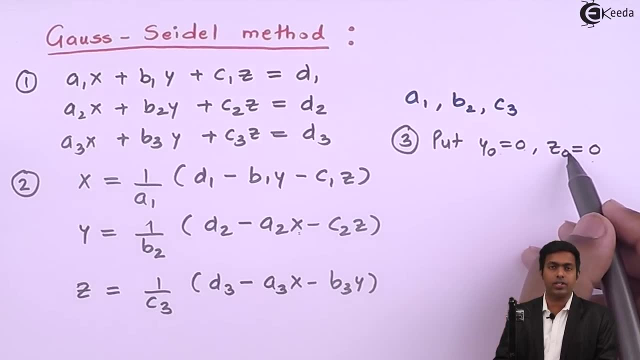 So we will get x2 because we got the recent or latest value of x as x2.. So x2 and z1 and we will go on. So by putting y0 equal to 0, z0 equal to 0, initially we will get value of x1.. 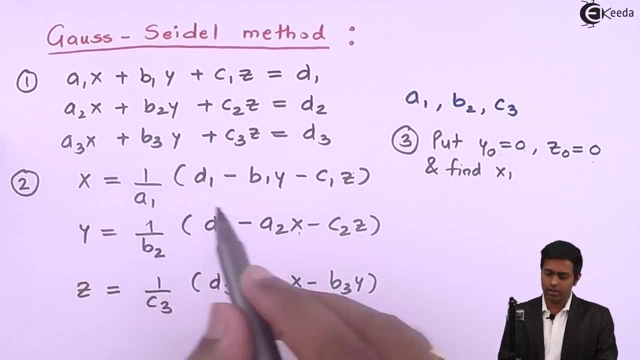 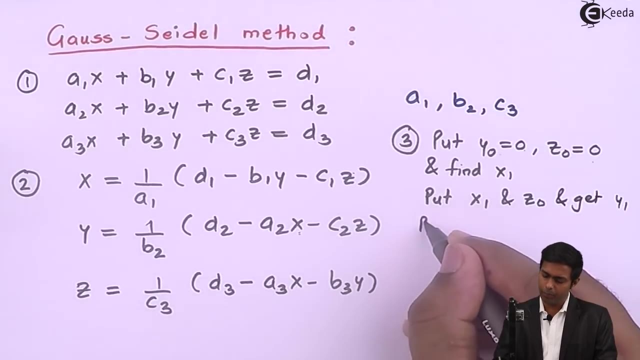 So here I will say: and find x1.. Once you get x1, here I will say: put x1 and z0 here and get y1.. Next, put the value of y1 and x1 and get z1.. So this is the first iteration and we will continue this iteration till we get the desired accuracy. 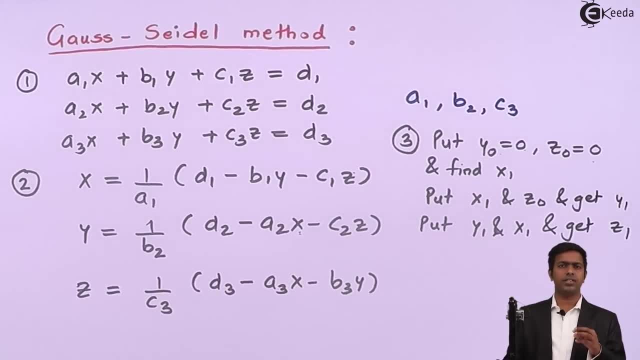 So whenever the values of two consecutive iterations are same, then that time we say that we got the desired accuracy and we stop the operation. And that is the value of x, y, z, or that is the required root of the equation. So to understand this concept, we will take one example. 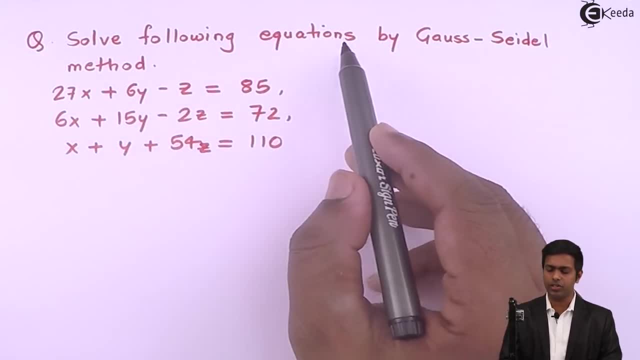 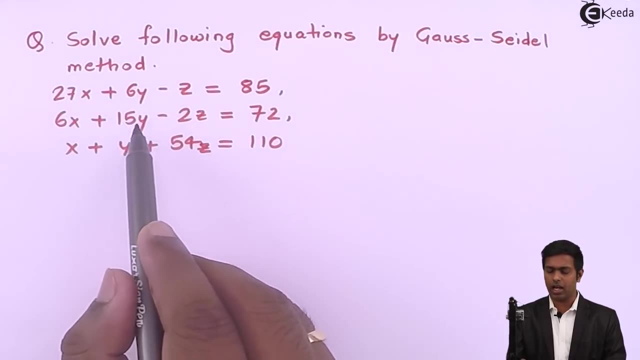 So the example is solve following equations by Gauss-Siedel method. So there are three equations and if you will observe, then see here these coefficients are large as compared to other coefficients. So we will convert these three equations in the form: 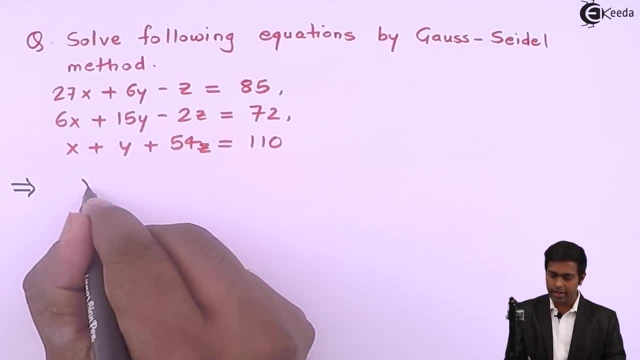 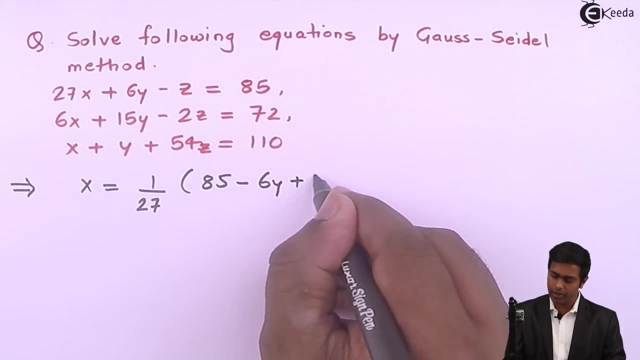 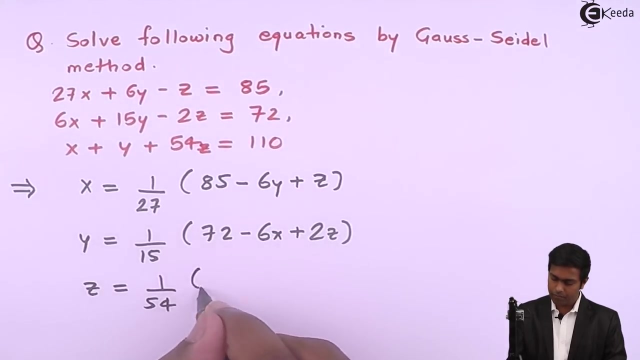 So here I will say: let x is equal to 1 upon 27,. 85 minus 6y plus z, y is equal to 1 upon 15, 72 minus 6x plus 2z, and z is equal to 1 upon 54, 110 minus x minus y. 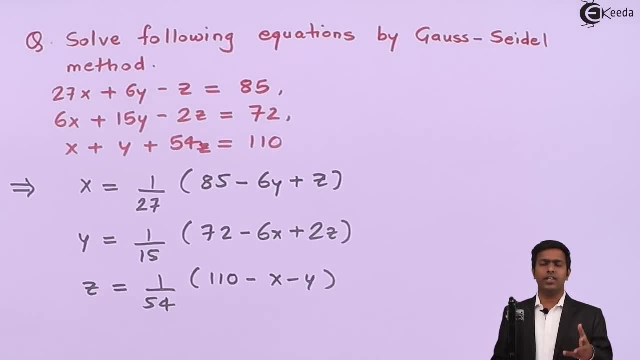 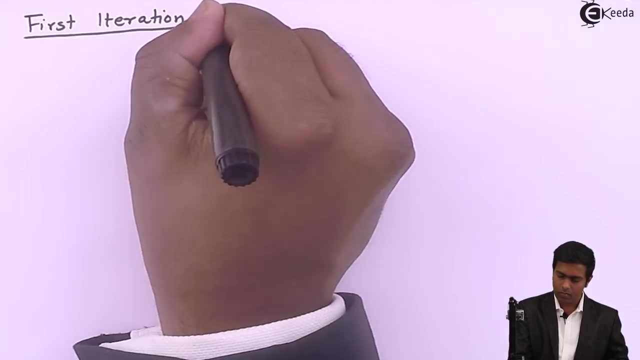 Now, here we got the value of x, y, z. Now we will start with the iterations to get the roots or the values of x, y and z. So we will start with the first iteration. Here I will say first iteration and here we will put y0 as 0 and z0 as 0. 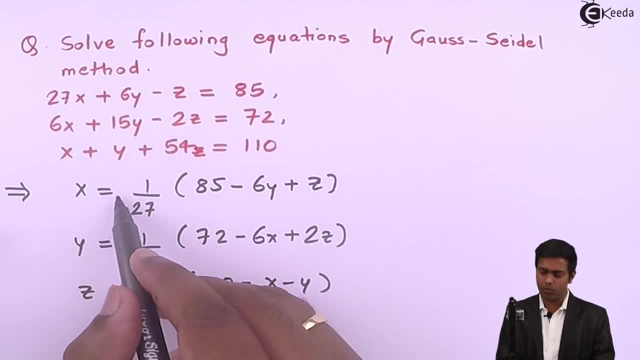 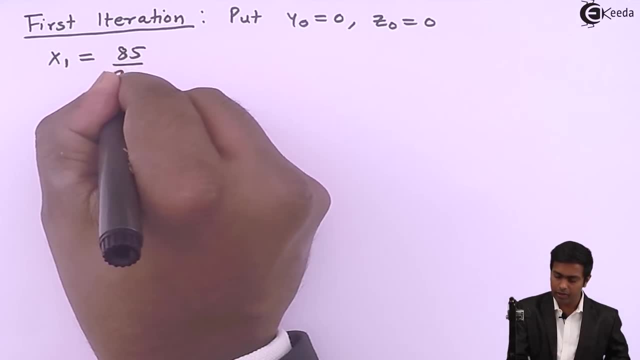 So by putting this over here we will get: x is equal to 85 minus 6y. So y0 is equal to 1 upon 25 and I will call it as x1.. So it is 85 by 27.. 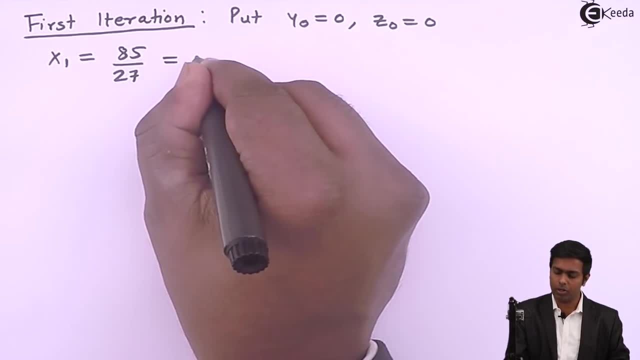 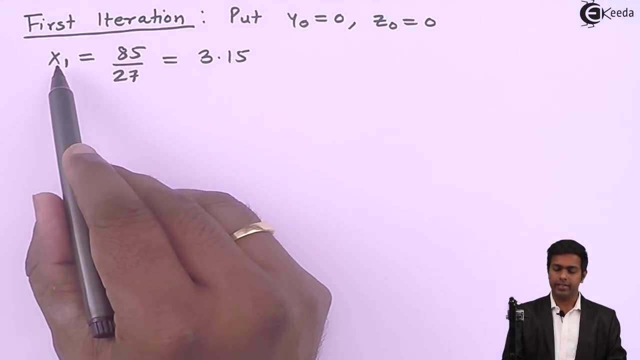 So in calculator, if you will check, then the value will comes out to be 3.15.. Now, as we got the recent value of x as x1, we will use this value in the next calculation to find out y1.. 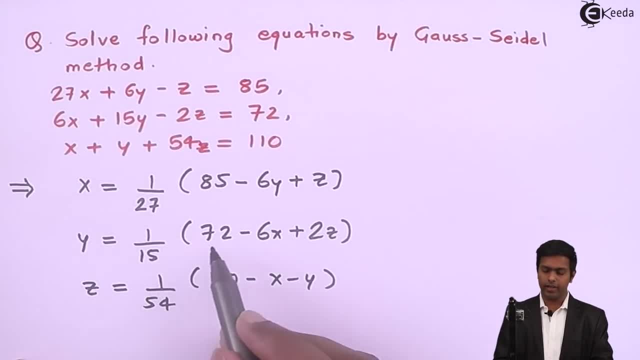 So the formula for y1 is 1 upon 15, 72 minus 6 times x1 plus 2 times z0, because the recent value of z is z0. So z0 is 0. So we will get 1 by 15, 72 minus 6 times x1. 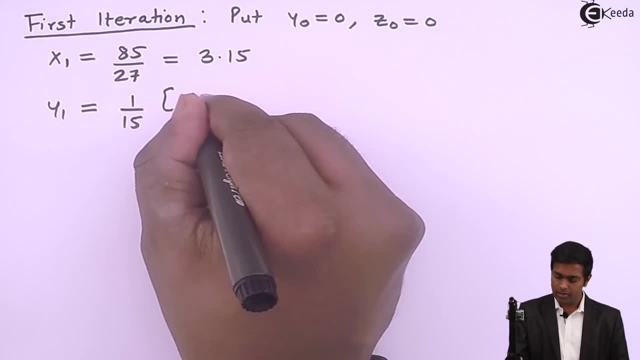 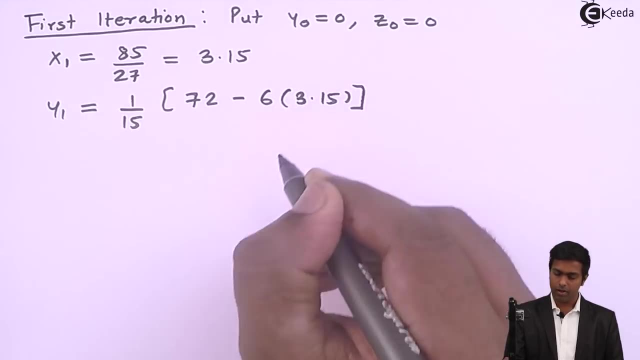 So here I will say: 1 by 15, 72 minus 6 times x1, that is 3.15.. And if you will check this in calculator, then you will get 3.54.. So now this is the recent value of y1.. 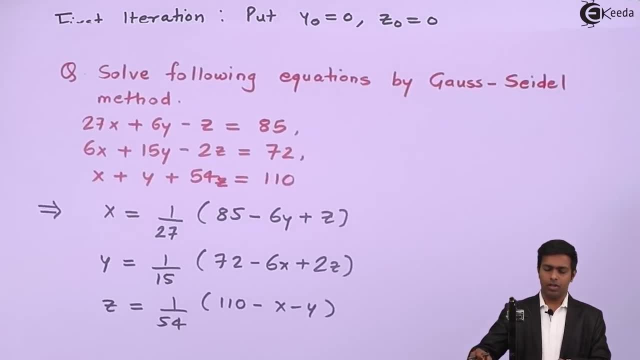 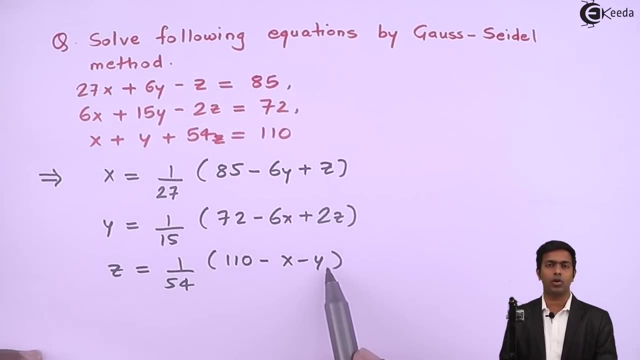 So z1 is given by the formula 1 by 54,, 110 minus. Now here I will use the value of x1 and y1 because they are the recent value, So 110 by 54 minus x1, minus y1.. 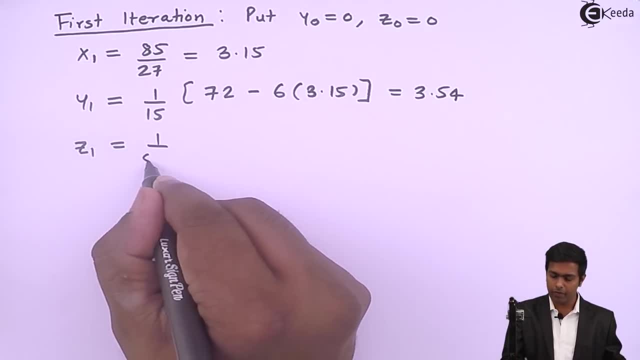 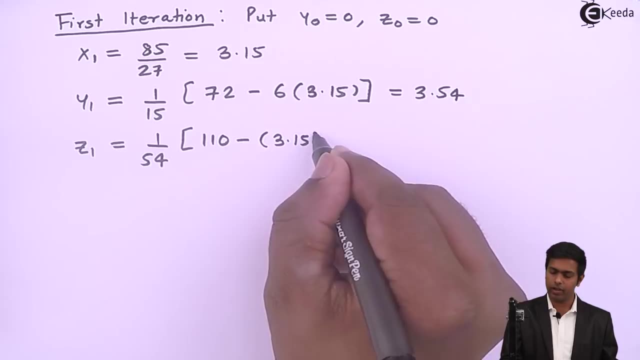 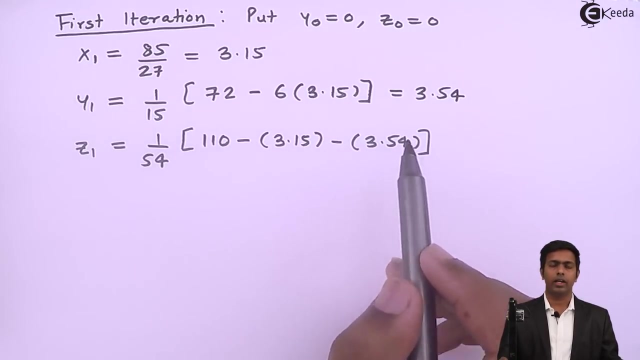 So here I will say: 1 by 54 in bracket, 110 minus x1, that is 3.15, minus y1, that is 3.54.. Now if we will calculate this value in calculator, then we will get it as 1.91.. 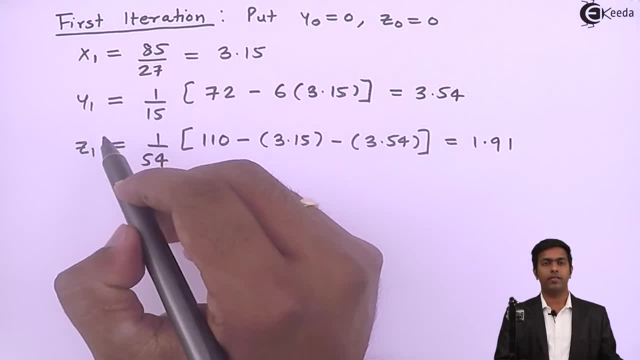 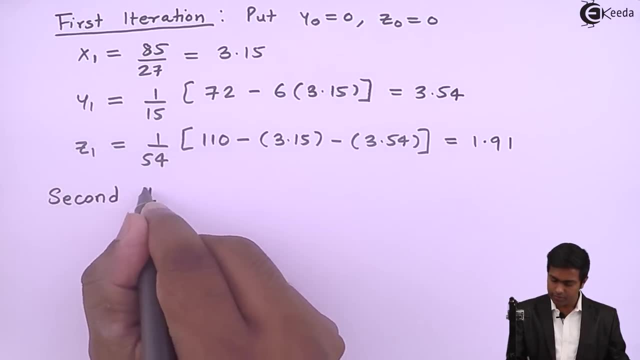 So now here we got the value of x1, y1 and z1. So we will move to the second iteration. So second iteration is So in second iteration we find the value of x2, y2 and z2.. 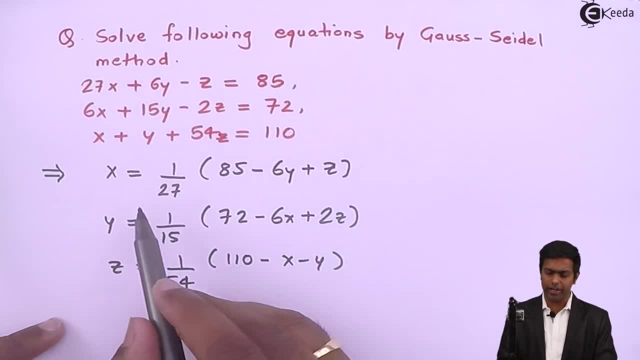 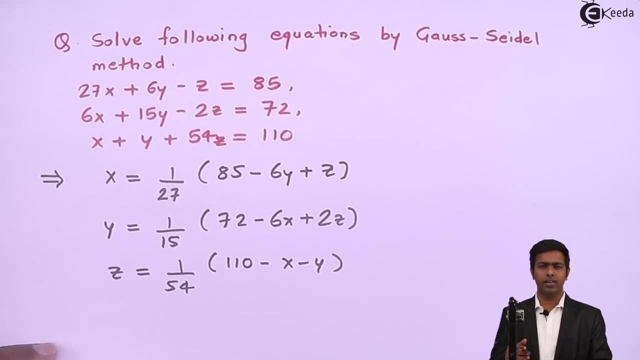 So, if you will see here, then to get the value of x2, we will need the value of y1 and z1 or the recent value of y and z, And here the recent value of y and z is y1, z1.. 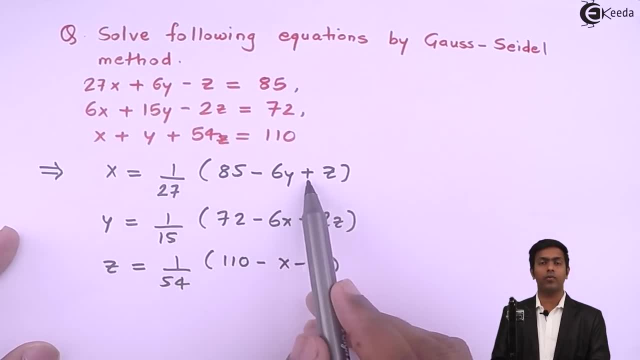 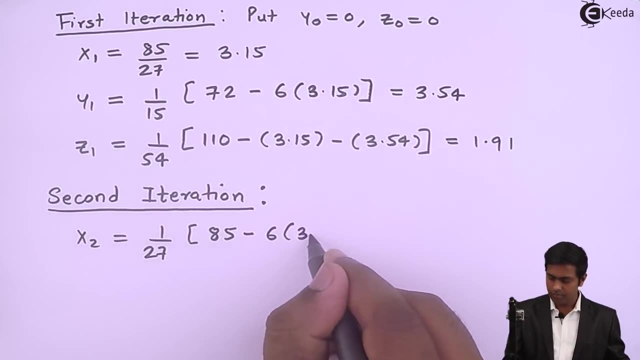 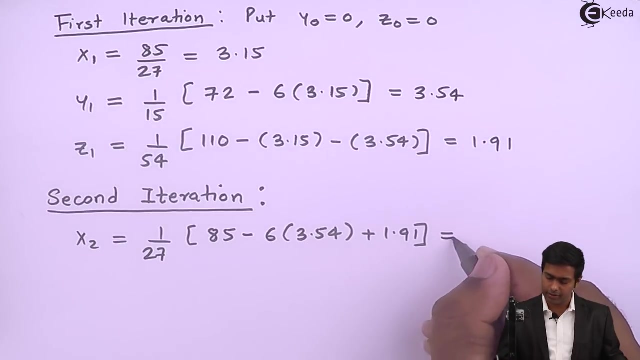 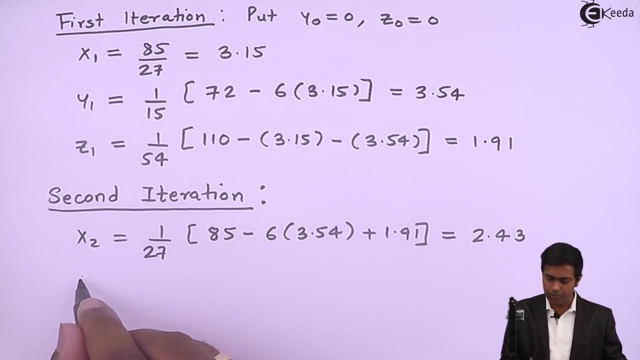 So here this formula will be 1 by 27 into 85 minus 6y1 plus z1. And it will become: Now, if we will calculate this in calculator, then we will get 2.43.. Now let us find out the value of y2.. 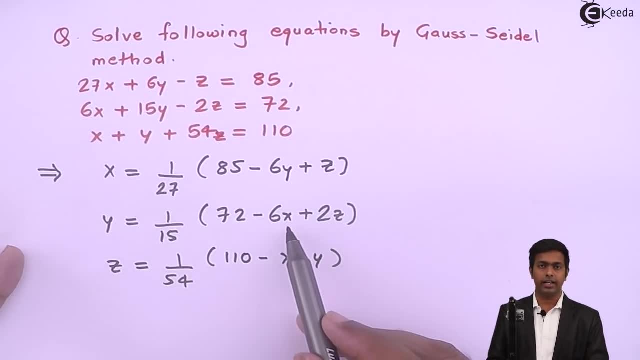 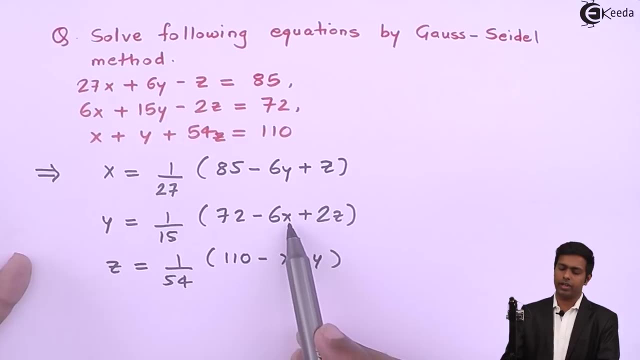 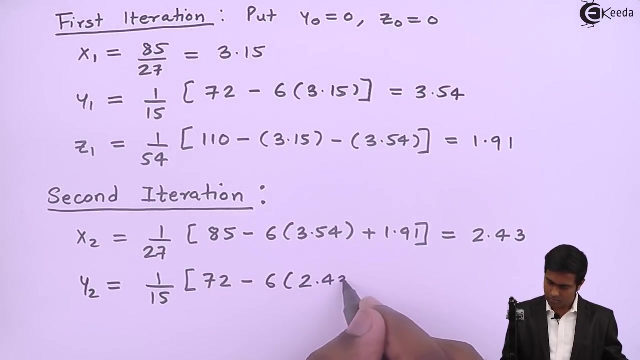 So for y2, we will consider latest value of x, that is the x2.. And the value of z as z1. So here x2 and here z1. So we will get. Now, if we will calculate this in calculator, then you will get. 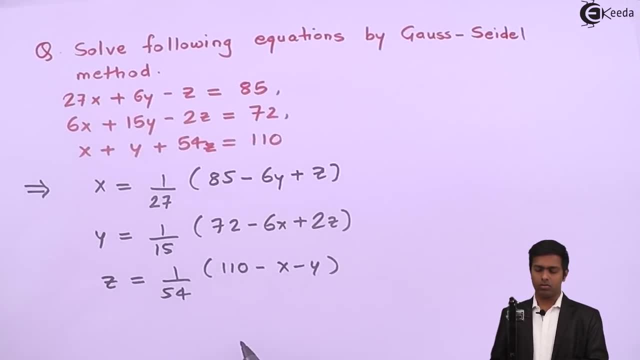 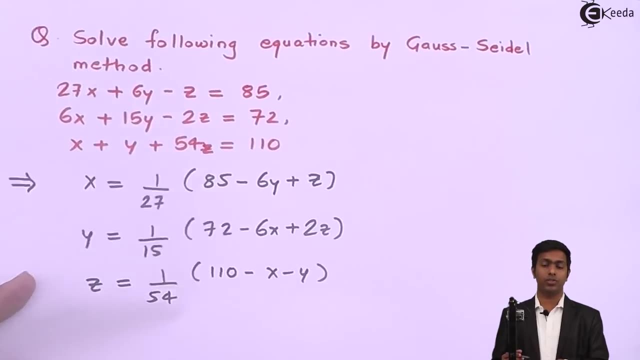 Next let us find out the value of z2.. So z2 will be 1 by 54,, 110 minus. Now, recent value of x and y are x2, y2.. We will use it there, So z2 is. 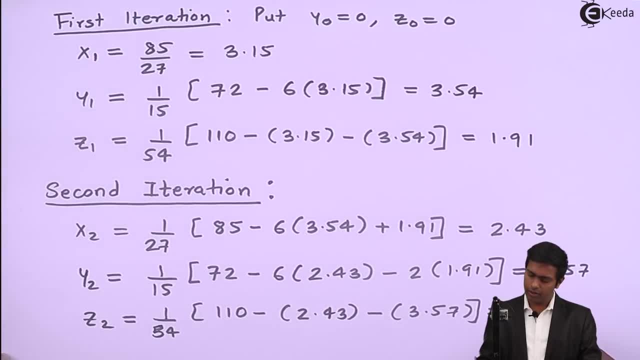 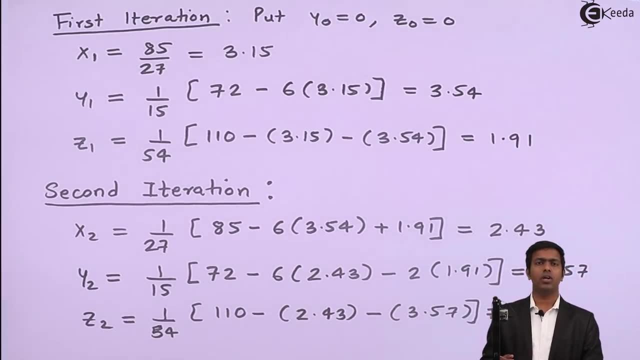 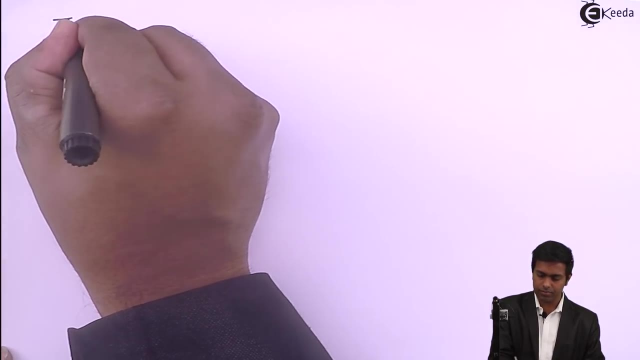 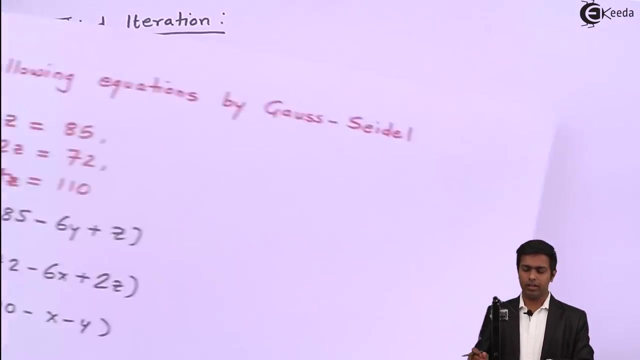 And this will give us 1.93.. So here we got the value of x2, y2 and z2.. Now we will use this value in the next iteration. So here I will say third iteration. So now for third iteration. we will refer the equations. 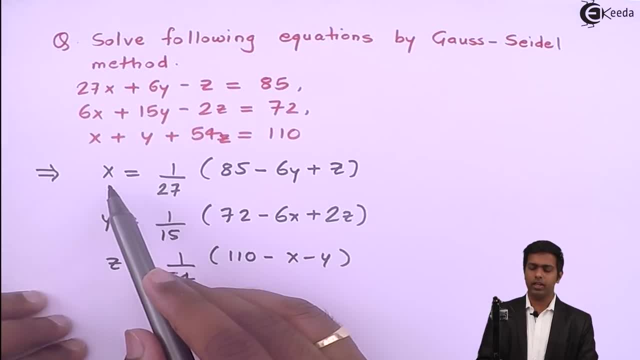 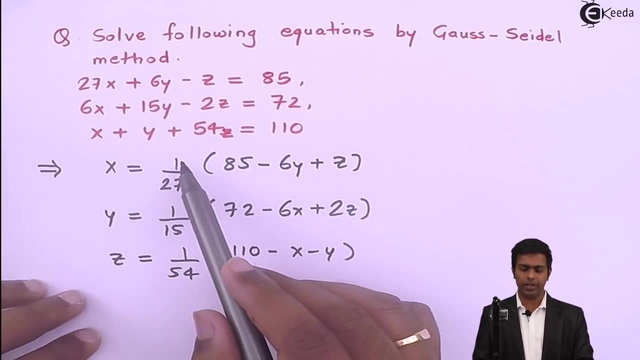 So to get the value of x3, we will use the latest value of y and z, And the latest value of y and z is y2 and z2.. So this equation will be 1 by 27, 85 minus 6 times y2 plus z2.. 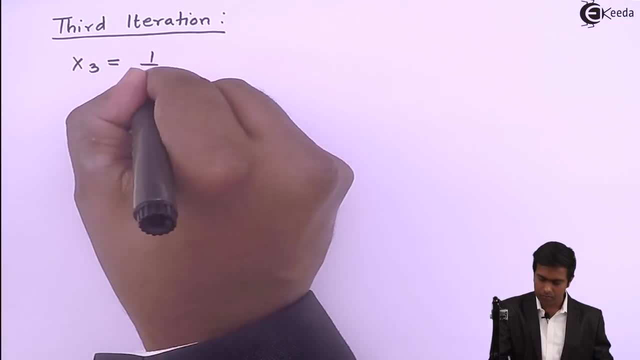 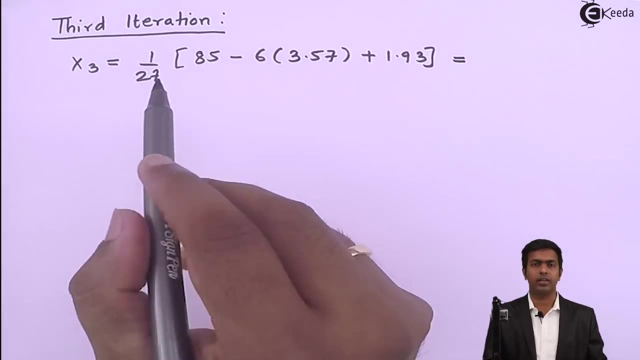 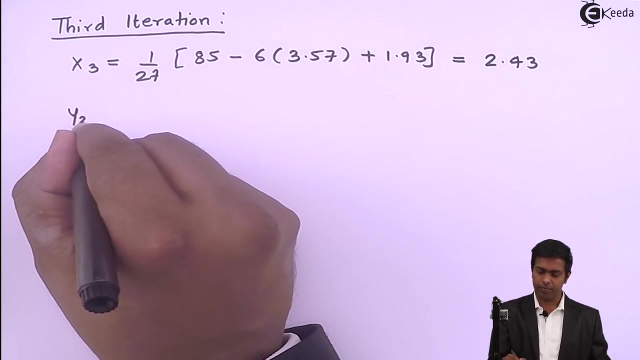 So this will become Now. if we will calculate this in calculator, then you will get- Now let us find out- the value of y3.. So if you will see here to get y3, we will use the latest value of x and z. 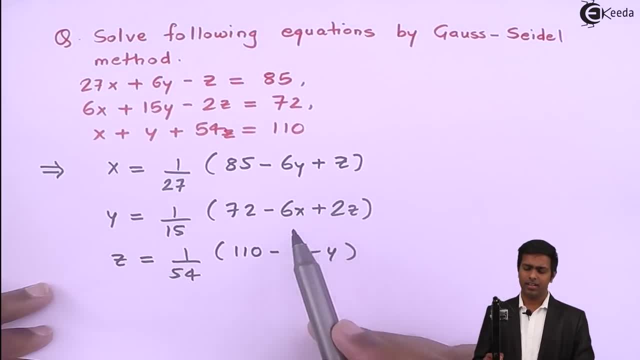 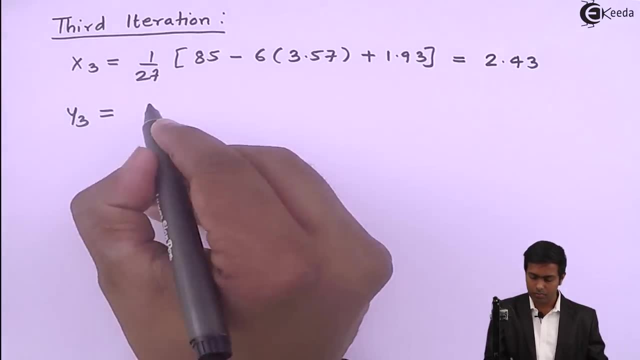 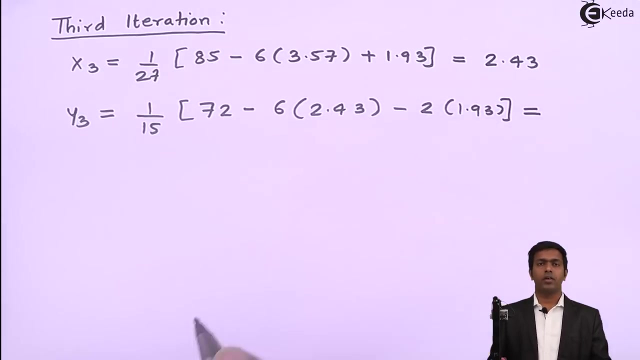 So the latest value of x is x3 and the latest value of z is z2.. So I will use value of x3 here and the value of z2 here. So we will get. Now, if we will calculate this in calculator, then you will get. 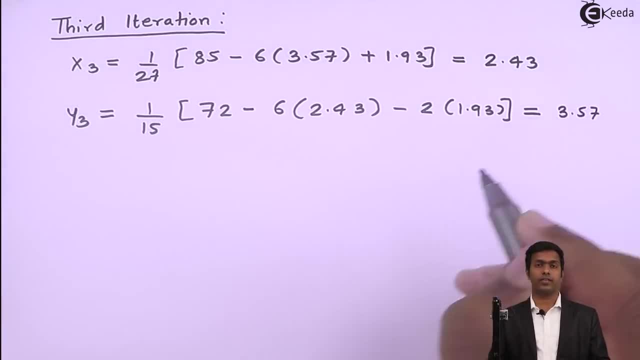 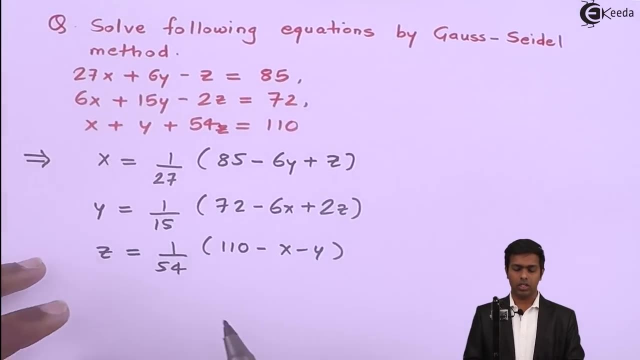 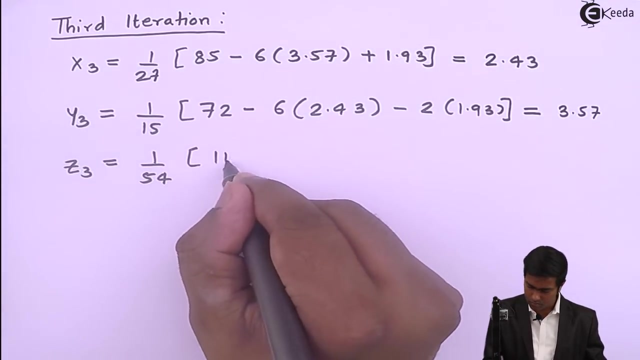 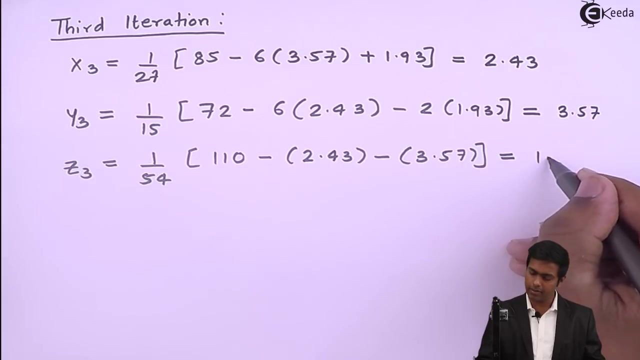 You will get 3.57.. Now let us find out z3.. So here to get z3, we will use the recent value of x and y, that is, x3, y3, and we will get. So here we will get 1.93.. 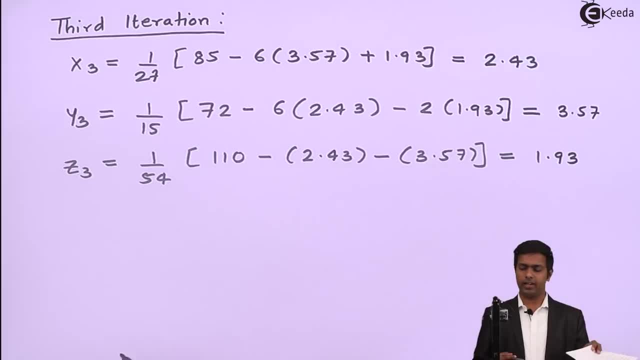 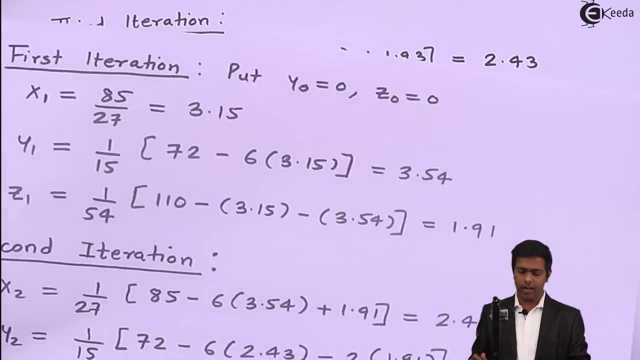 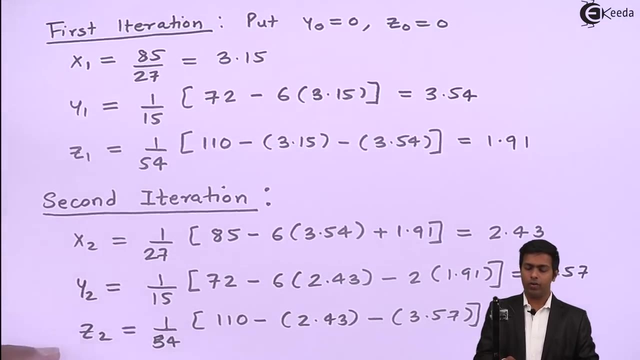 Now, if you will compare this third iteration with second iteration, Then value of z3 is 1.93, whereas in second iteration the value of z2 is also 1.93.. Next, value of y2 is 3.57, value of y3 is also 3.57, and value of x2 is 2.43 and value of x3 is 2.43. 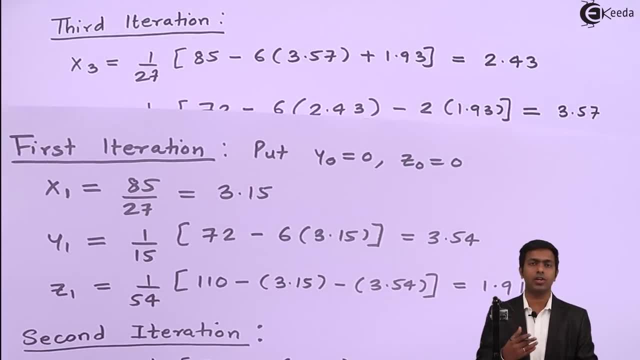 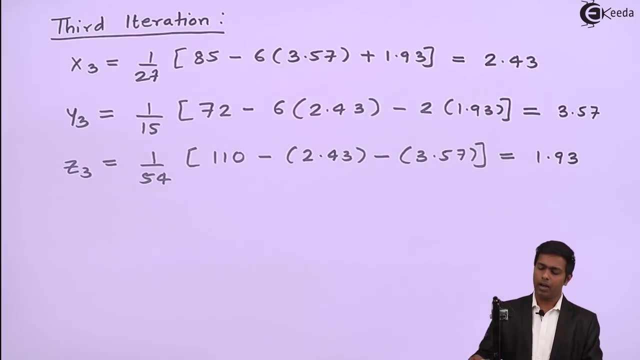 It means we are getting the same value in the consecutive iteration. So, as I said, that whenever we get the desired level of accuracy we stop And we call them as the roots. So here our roots are: x equal to 2.43, y is equal to 3.57 and z is equal to 1.93 for the given simultaneous equations. Thank you. 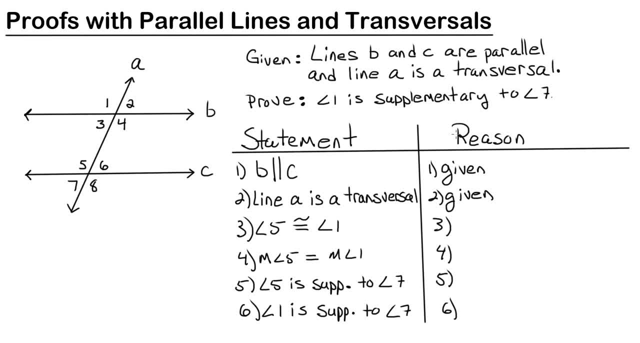 Alright, so let's take a look at some proofs with parallel lines and transversals. So, given lines B and C are parallel, here they are lines B and C and line A is a transversal prove that angle 1 is supplementary to angle 7.. So remember, supplementary means that they have a sum of 180 degrees. 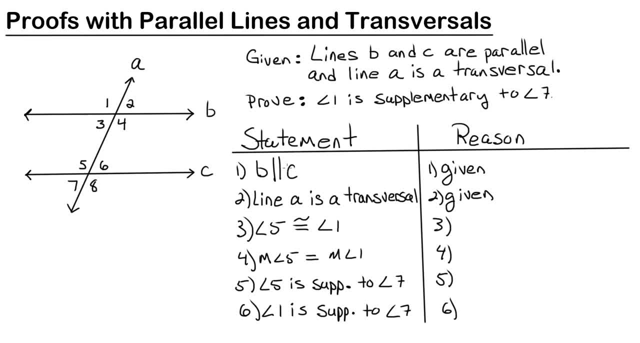 Let's take a look at our statements and reasons. So our first statement, B, is parallel to C. we know that because it is given. Our second statement, line A, is a transversal. we know that because it's given. 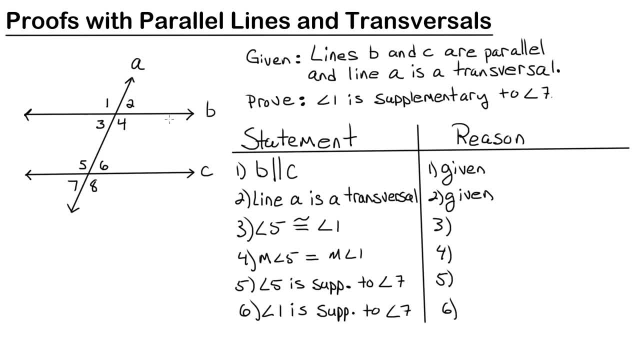 Looking at statement 3: here it says angle 5 is congruent to angle 1, we see here's angle 1, here's angle 5, they are both to the left of the transversal and on top of their lines, so they are corresponding angles. 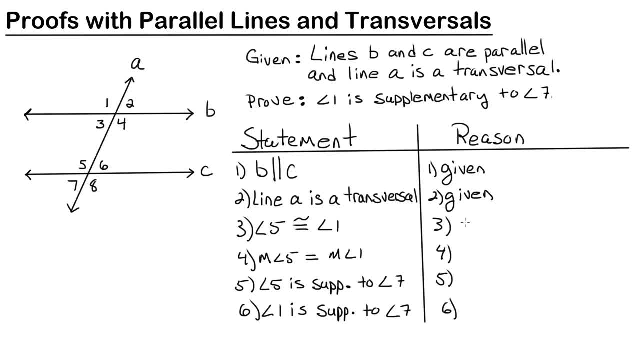 So we know that angle 5 is congruent to angle 1. Because of the corresponding angles theorem. So I'll just do this: for angles theorem, Statement 4, the measure of angle 5 is equal to the measure of angle 1, and since we know that they're congruent, that's how we know they're equal. so that is definition of congruence.